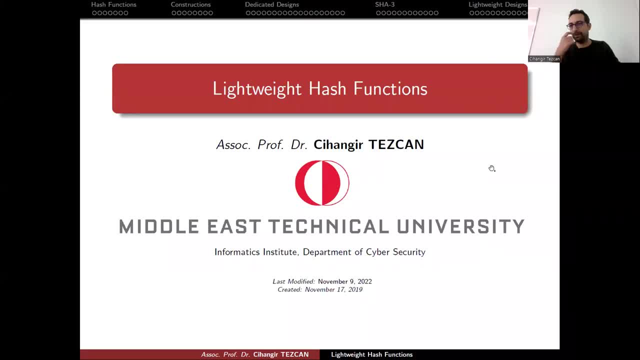 All right, so our topic is lightweight hash functions. but before talking about light hash functions, I have to describe what the hash function is. then we will talk about popular hash functions. then we will move on to lightweight standards. So let's start. 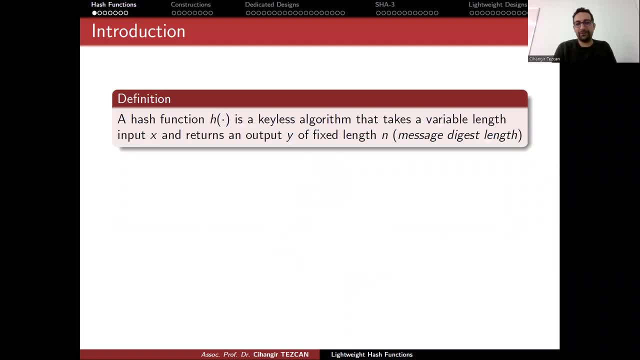 with the definition. first, A hash function H is a keyless algorithm that takes a variable length input X and returns an output Y of fixed length N, which we call message digest length. So the definition is really simple. Input size is variable, Sometimes it is infinite. 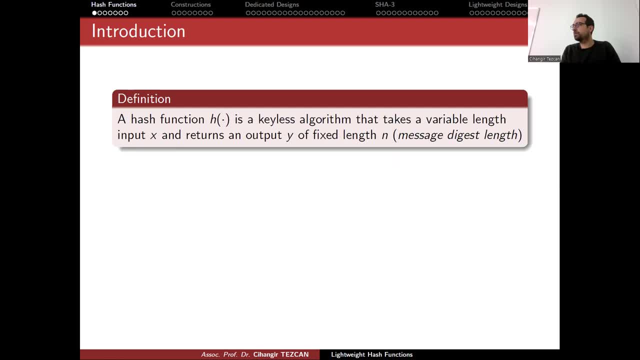 but in standards generally it is limited with 2 to the 64 bits, So virtually it is infinite. actually You would never have that amount of input, but the output size is fixed and sometimes it is 128 bits in older versions of hash functions. 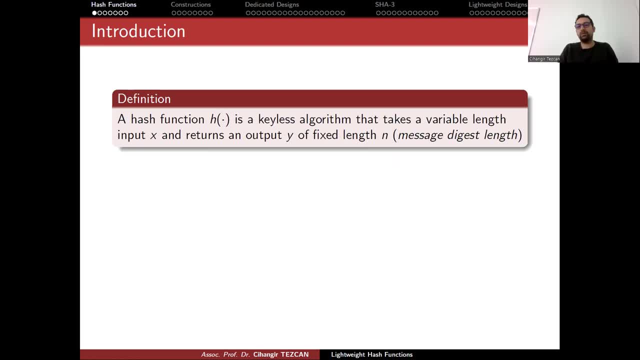 But in popular or modern hash functions the output N is 256 bits or, if you want, 512 bits and so on. So we have some standards in this. So when we say SHA-256, actually we are talking about SHA-2 algorithm, which has an output size of 256 bits. but that algorithm 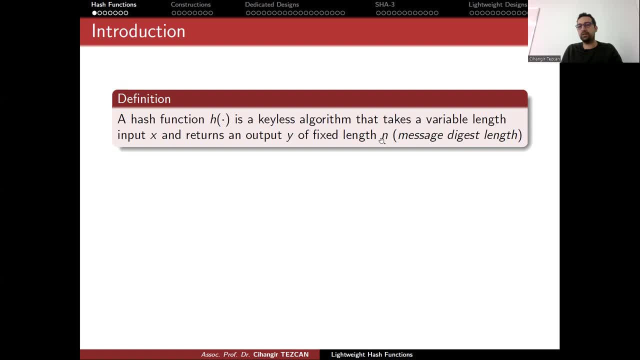 actually have four different output lengths, So it is up to the user to choose. Okay, But it is simple. The input is from a very huge space and we are mapping this very huge space to a very smaller space, which is also really big Because if it is N bits, 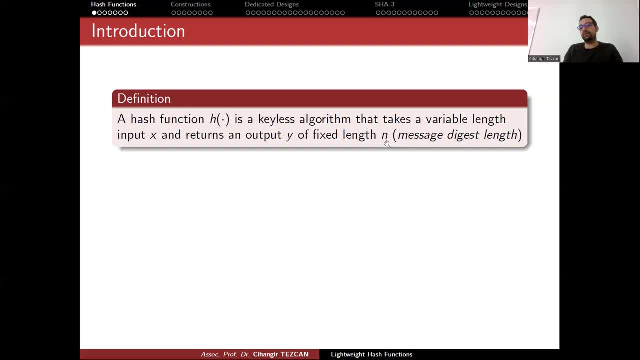 then it will be 2 to the N- many elements, right? And if you choose N256, then 2 to the 256, you know is around the number of atoms in the observable universe. So this definition of a hash function, but we are going to talk about cryptographic hash functions And from 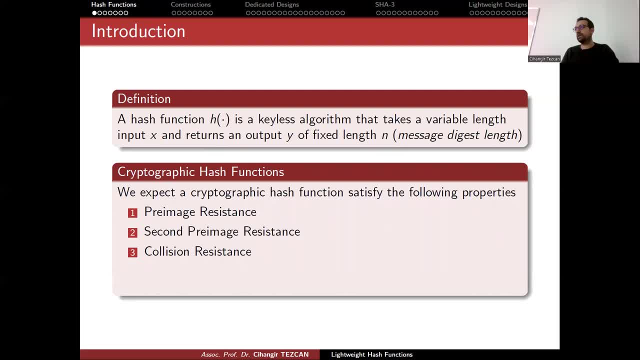 a cryptographic hash function. I want some properties. Okay, So we expect a cryptographic hash function to satisfy the following properties: These three properties called pre-image resistance, second pre-image resistance and collision resistance. Okay, I will explain all of them one by one. Moreover, since we are going to have an output of 256 bits, we also want to. 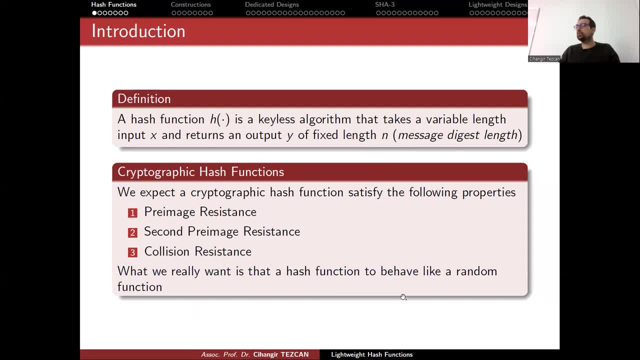 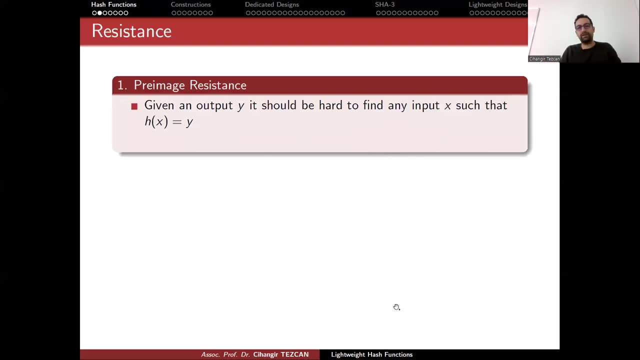 have that output to look like a random number. Okay, So what we really want is that a hash function to behave like a random function, And this is actually used in, you know, in many areas like cryptocurrency, mining and so on. But let's move on with the first property. So I said that. 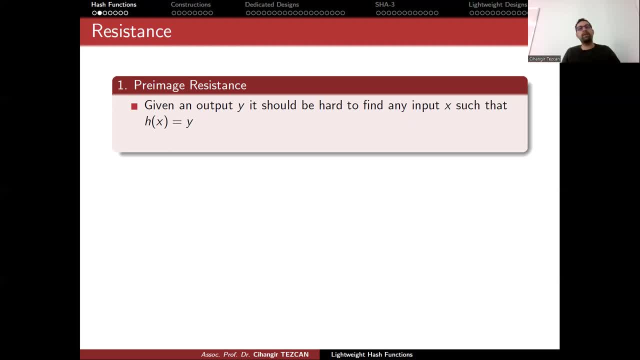 I want a cryptographic hash function to be pre-image resistant. This means that, given an output Y, it should be a pre-image resistant. So I want a cryptographic hash function to be pre-image resistant. This means that, given an output Y, it should be a pre-image resistant. So I want a. 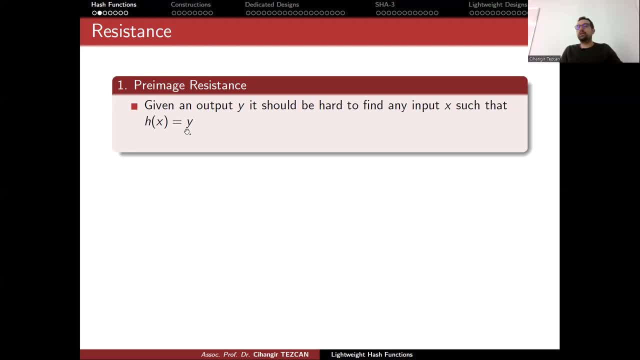 cryptographic hash function to be pre-image resistant. This means that, given an output Y, it should be hard to find any input X, such that HX equals to Y. Okay, So I am saying any because, as you notice, the input space is a lot larger, but the output space is fixed to the two, to the N bits, right? 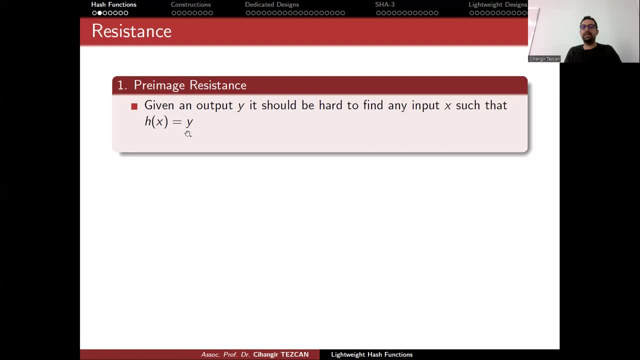 So more than one input will give the same output. But here the question is: for instance, I'm choosing an X and calculating the output, And now I'm giving you the output and asking you: can you find any input that gives you this output? So this hash function generally. 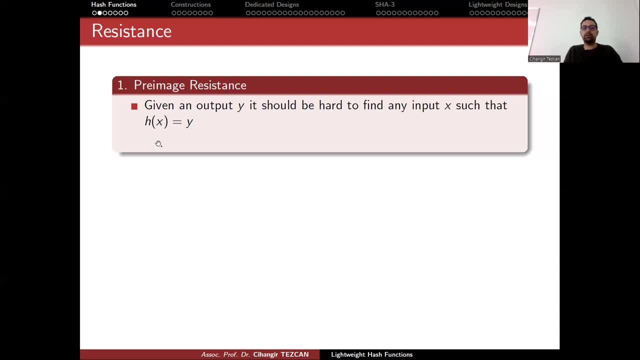 sometimes it's called one-way function. So you know the algorithm definition. So when you have the input, you can easily calculate the output. Okay, Question is: once you know the output, can you find an input that gives you this output? So we want this to be hard, But of course, 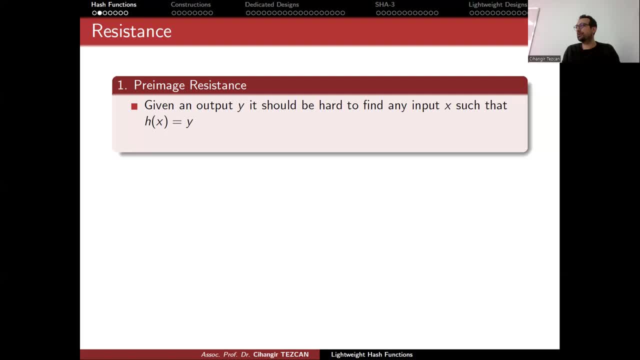 here. hard is not a scientific term, So actually we wanted to. we saw secure that a generic attack, which means that trying every X, one by one, will require around two to the N operations. Okay, And since N is big in our scenario, like 256, so a brute force attack. 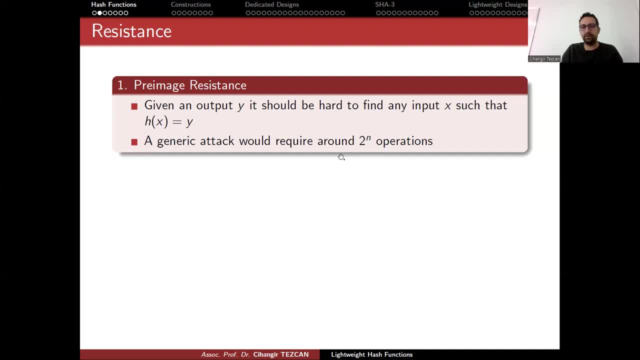 should take a lot of time. Currently, it is not possible to perform this many hash operations. So you might ask, why would we require such a thing? Actually, we required for many reasons, but I will give you one example. So in the 1990s, what happened is that when you created a password, it was not possible to perform this many hash operations. So you might ask, why would we require such a thing? Actually, we required for many reasons, but I will give you one example. So in the 1990s, what happened is that when you created a password, 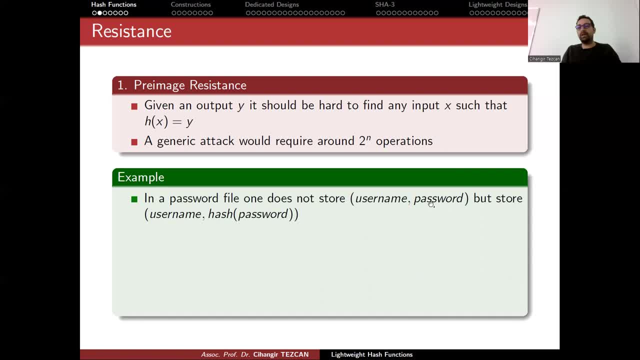 in a web page so they start their username and password in the database in the same tables. okay, as a plain text. So your username and password. So a lot of databases leaked in the past and all of these companies become bankrupt and you know they have to close down Because once the database leaks, all of your passwords leaks, right. So since your username is also there, now unauthorized people can't log into your account, and so on. So basic a way to overcome this problem was to store username and hash of the password. 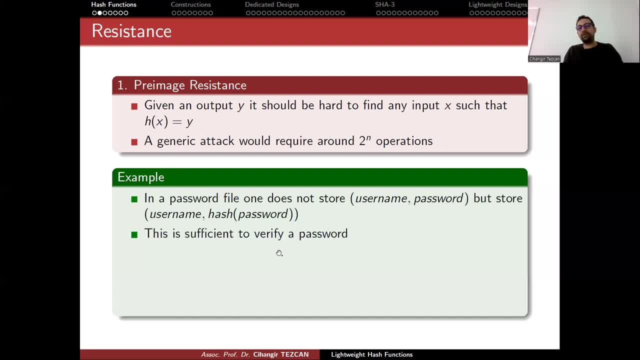 not the password itself. okay, This way this is sufficient to verify a password, because they are storing your hash value. So whenever you want to log in, you provide your password again, they calculate the hash of it and check if it matches with the one in the database. So this way, 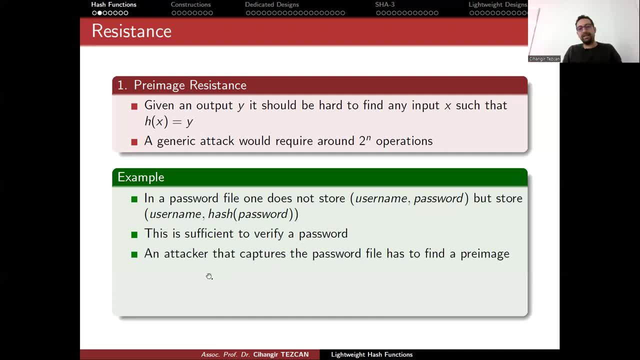 this is enough for them to authorize you, And an attacker that captures the password file or the database table has to find the. pretty much because now they have the hash value, But in order to log in they have to know the passwords. Okay, so from why they have to come up with the next? okay. Of course, if I stop here, people might 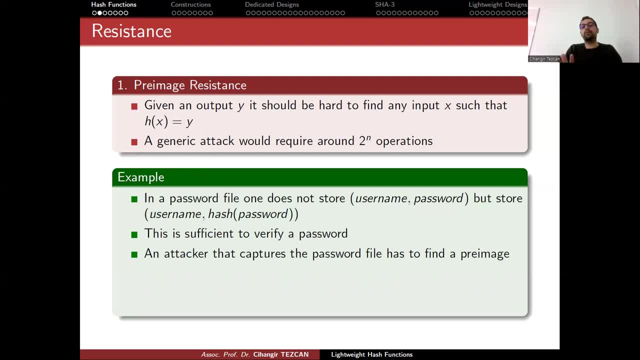 think that this is how you store a password, But this is not enough. What we do in practice is as follows: We also concatenate a random value called salt, sometimes 32 bits, sometimes 64 bits, And so, instead of your password, you concatenate a salt value to end of it. 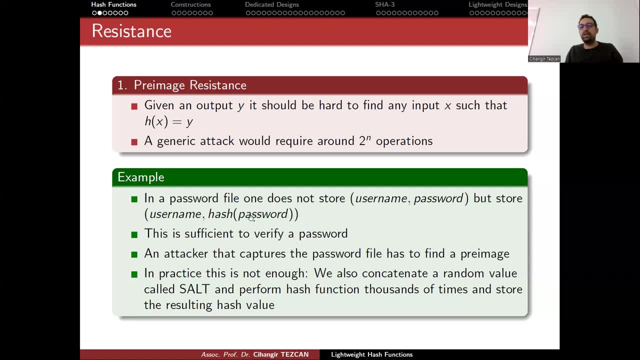 Then take the hash value, calculate the hash, but do not stop here. Take the output and put it as if it is the input of the hash function. obtain another output, put it as an input, and so on thousands of times, And after that maybe 10,000 times. 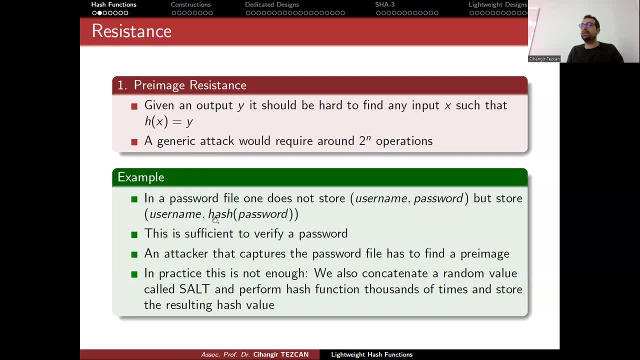 later you obtain a value and store only this value in the database. Okay, you might think why this is the case. I'm putting the salt value there to prevent dictionary attacks, because a lot of people, if you store it like this, they. 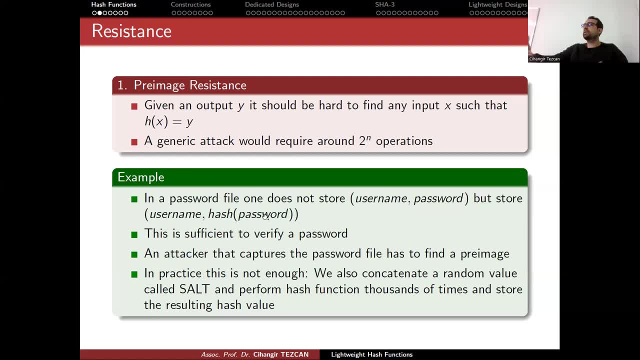 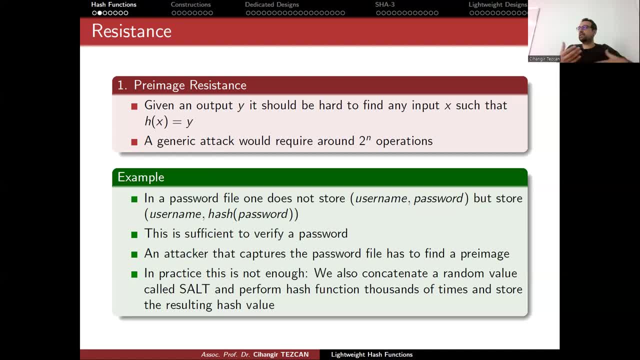 database leaks, they will check their dictionary and they check if any of them matches with the hashes of the passwords of the inside the database. So salt prevents the dictionary attack, But this doesn't prevent the brute force attack, Because if you add on the salt to here, so whenever database leaks, since the salt values, 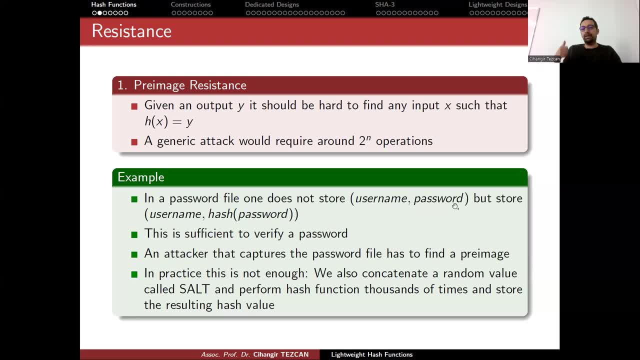 also should be included in the database. hacker now knows the hash value and also the salt value, So they can try every password one by one. So if you have a weak password, their brute force attack will be successful. So, in order to slow down, 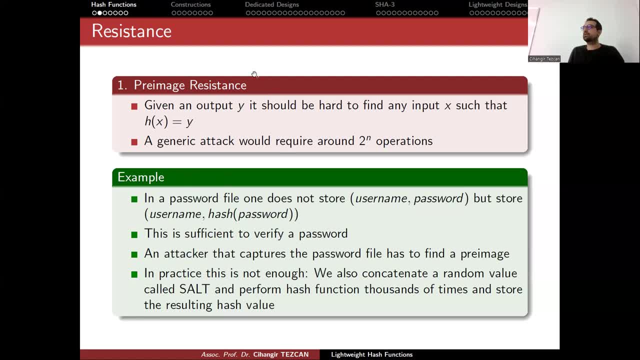 this attack. this is why we are performing this hash function thousands of times. So when you want to log into a web page, you provide your password. So they have to calculate their hash value of your password, maybe thousands of times times, but this is done in milliseconds so you will not feel any difference. but when the hacker 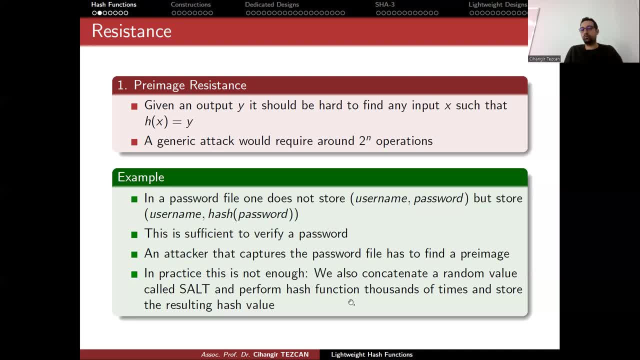 wants to try every password. so if you chose the number of hash function usage as 10 times, 10 000 times, this means that you slow down the attacker 10 000 times. okay, this is how you should store a password, okay. or you can even choose a- instead of a hash function, a dedicated function. 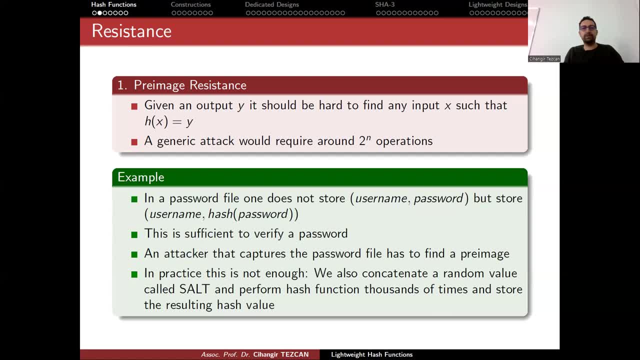 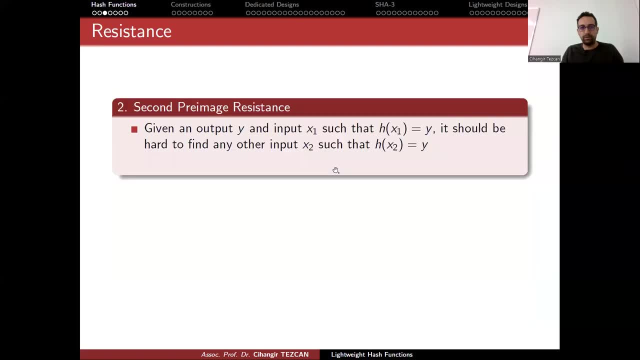 for password hashing and there was a competition about it, but no one knows about it yet. okay, so let's move on to the second part. this property is called second primary resistance. so given an output y and an input x1, such that h x1 equals to y, it should be hard to find. 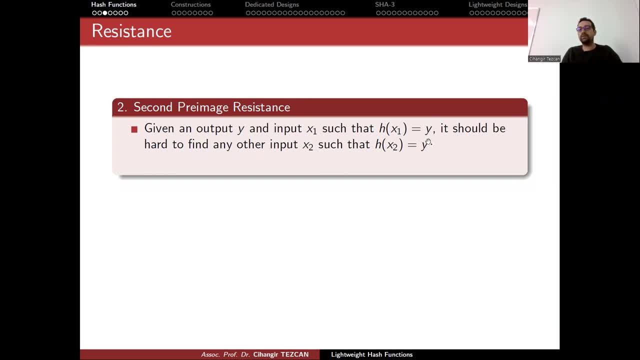 any other input x2, such that hx2 also gives the same y. okay, so this is called second pre-image resistance. again, you can try to perform a brute force attack. you know, put, try everything and expect to come up with some y. but since y is m bits, a generic attack would. 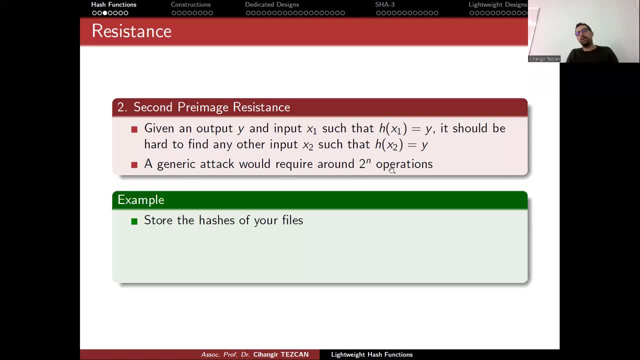 require two to ten operations. okay, so why do i require this? actually, uh, almost every cryptocurrency that uses blockchain, you know uh is secure due to this property. otherwise, you know you might say that, okay, everything inside this block gives this value. but actually it was something different. if you provide the same output, you might say that, okay, the transactions were different and 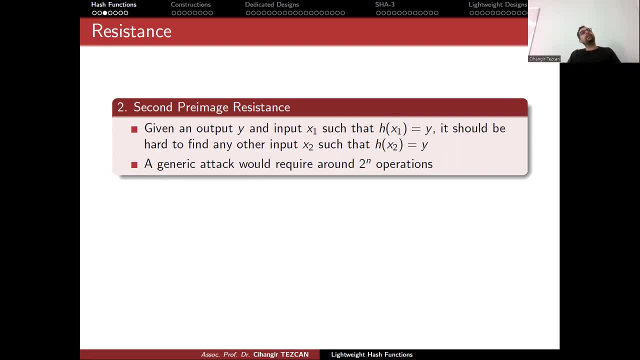 the correct transactions were like this, or as a easier way to explain: for instance, i'm sending you 1000 turkish liras, okay, and i'm digitally signing it, but you don't sign the message itself, you sign the hash of it. so i'm signing y saying that this is what i have done. so if you 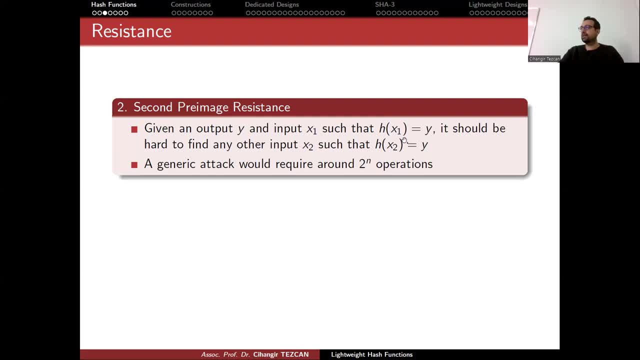 go and provide x1 which tells that i'm giving you 1000 turkish liras, the- i will not deny it because i signed this right. but if the hash function is really bad and if you can come up with x2 which says i'm giving you 1 million turkish liras but the output is still y, since 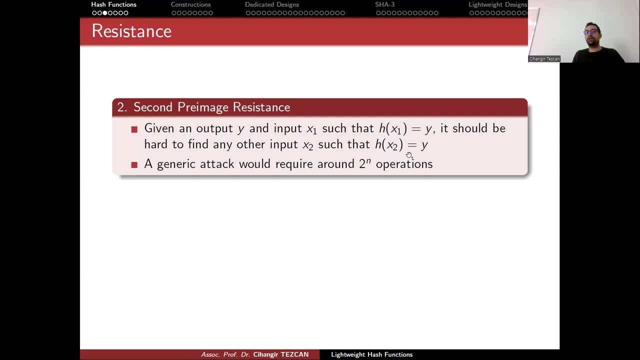 i already signed this message. this means that i also signed this one, so you can provide x2 instead of x1 and claim that i owe you 1 million turkish liras. okay, so for digital signatures. second, pre-image is really important, but another way to you can use it sometimes. i suggest it to people who are 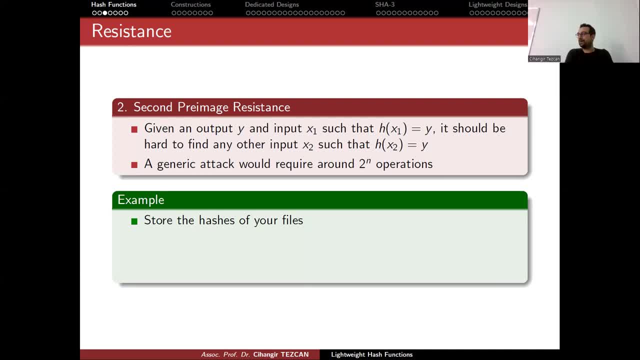 paranoid. store the hashes of your files. okay, keep them in a table, in a different drive. and because some people think that maybe there is a virus inside the computer and maybe some of the files are changed, how would you know? right? so store the hashes of your files if the attacker modifies the. 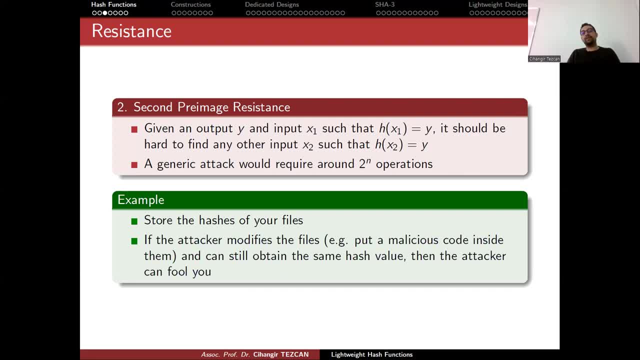 files, for example, put a malicious code inside them and can still obtain the same mesh value. the attacker can fool you, right. but from a good hash function, if it is second pre-image resistant, this cannot be done. so if you store all of your hashes, then you can say that, okay, this file is. 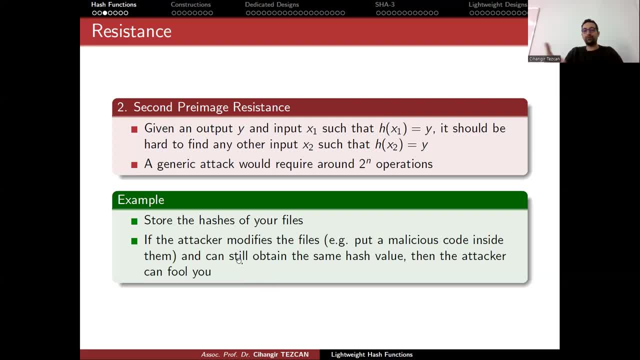 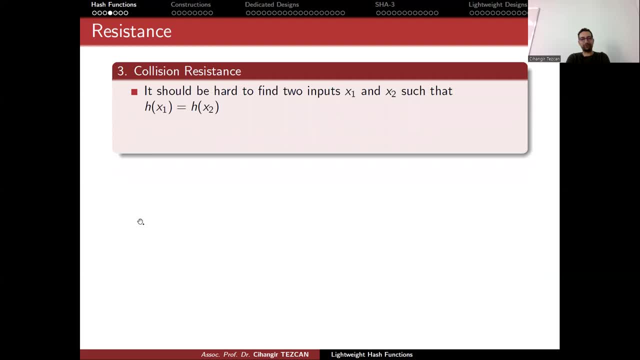 now modified. okay, if you're paranoid, you know, write an automated tool which checks all of these hashes. you know, from time to time it should be nice homework actually. so the third property: it should be hard to find two inputs, x1 and x2. size that h. 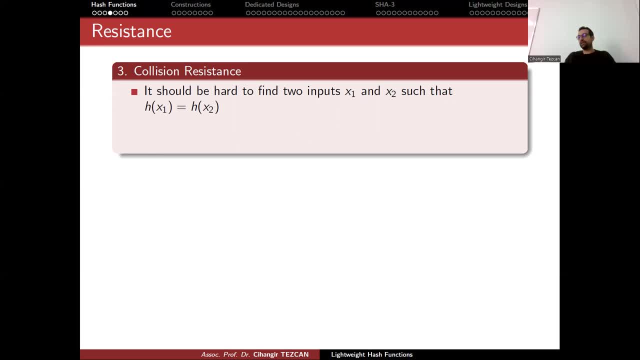 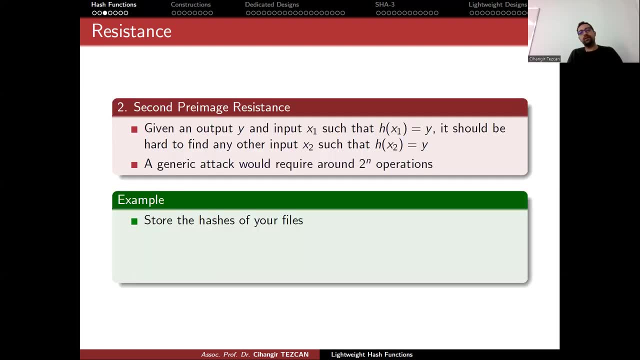 x1 equals to hx2, which equals to some y. so you might say that what is the difference of this one with the previous one? but if you go back to previous one, in this scenario x1 is fixed. i'm giving you x1, i'm giving you y and asking you to find x2. now we have more freedom because i'm only 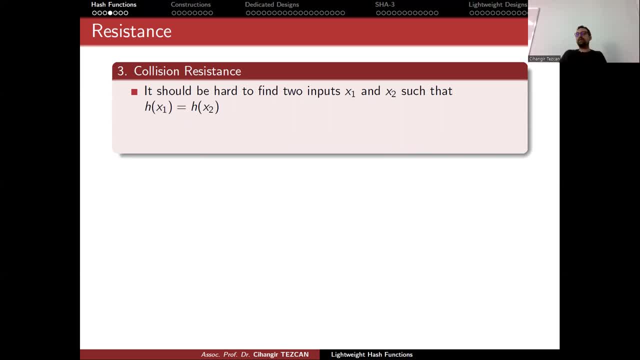 giving you a hash function and asking you to find two inputs that give the same output. so you have more uh freedom here. okay, so a generic attack now would require, instead of two to the n, like in the previous properties, now it requires square root of it, which is two to the n over two operations. 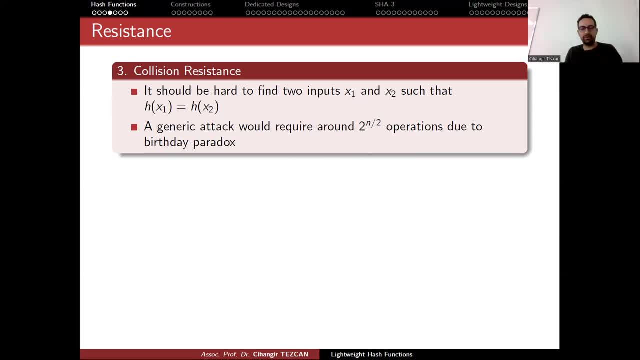 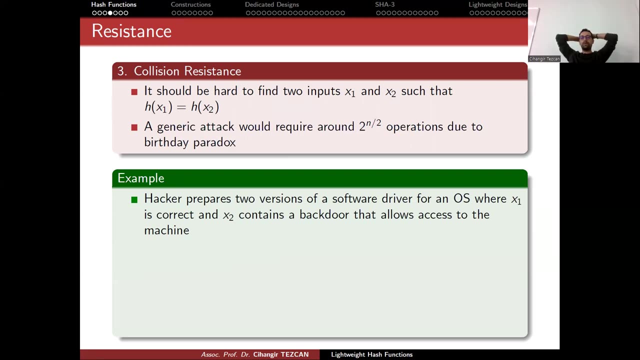 due to birthday paradox, which i will explain in the following slide anyway. so it is easier to find collisions than you know finding pre-images or second pre-images. so how can you use this? so if you have control over both x1 and x2, a hacker can do the following: a hacker prepares two versions of a software driver for an operating. 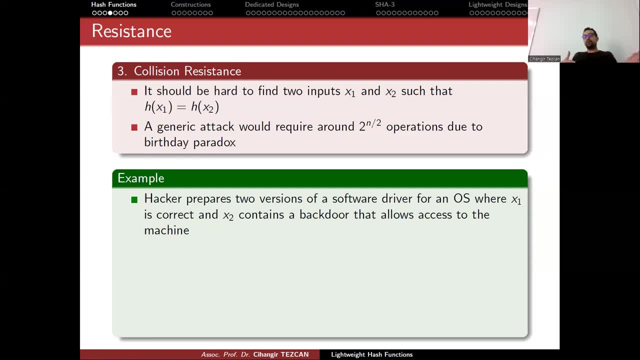 system where x1 is correct and x2 contains a backdoor that allows access to the machine. okay, so hacker sends x1 to the operating system company for inspection. they check it, they find no problem and they signs the hash of this x1. you might say that why they don't sign the whole? 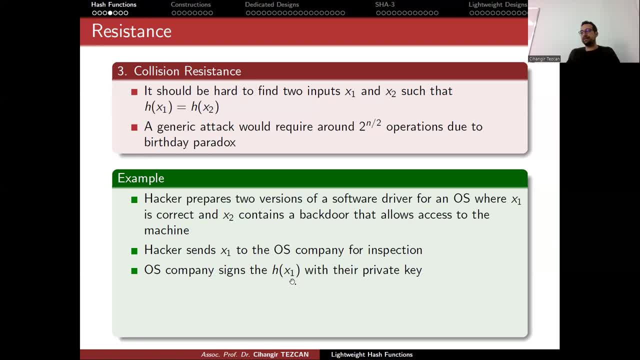 driver. but nowadays, you know, sometimes drivers even exceed one gigabyte of data. you cannot sign something that big and the data size increases. when you sign something okay, even if it is one megabyte, once you sign it it will be larger, so this is why we sign the hash of it okay. so now, since they signed the hash of this image x1, sorry, 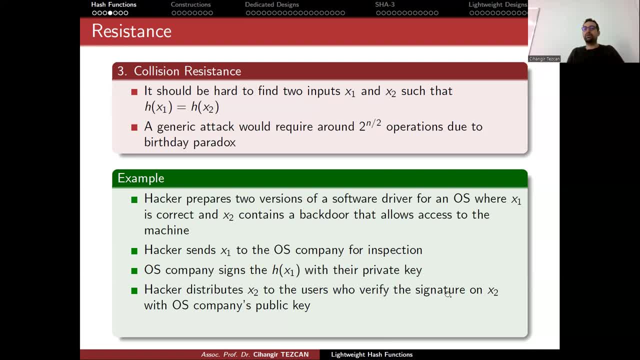 hacker now distributes x2 to the users who verify the signature on x2 with the operating system companies publicly. so since you distribute x2 when anybody wants to install, this driver operating system will calculate the hash of x2, which will be the same as this one, and check that their signature is. 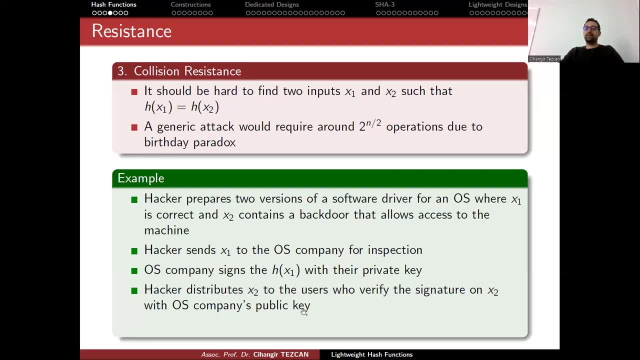 correct. so they will verify the signature and they will say that the operating system, that this is digitally signed. so this driver is secure, but actually it contains a backdoor. this works because you know we said that h x1 equals to h x2. of course, this is not something. 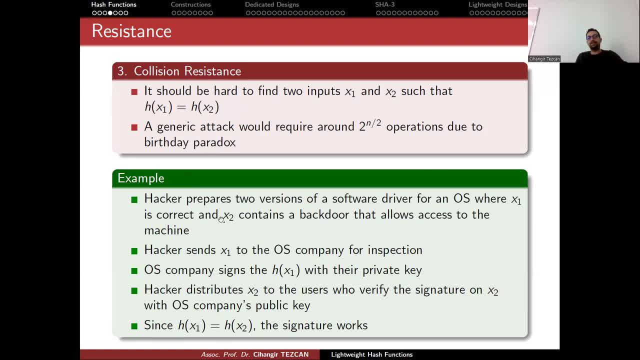 easy to do because coming up with the same you know driver with one of them having a virus, the other one does not, but still provide the same hash value. so it is something hard. but flame malware did this years ago with md5 fresh function okay, so it can be done. let's look at the birthday paradox, because 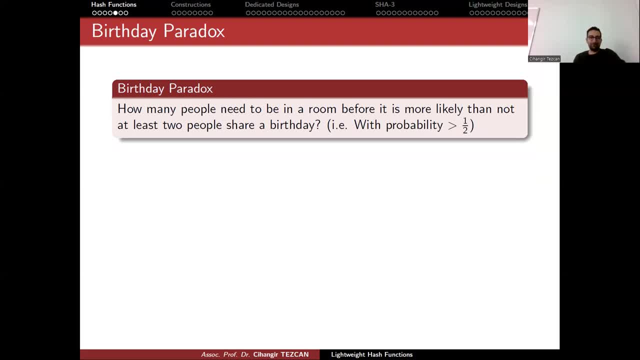 the name has paradox in it. people like this, so we have to talk about it. so question is: how many people share the same birthday to the other person? so let me go to this example here. so we have to take a look at the birthday paradox. so it will be basically a day of our birthday. it is likely to be in a room. 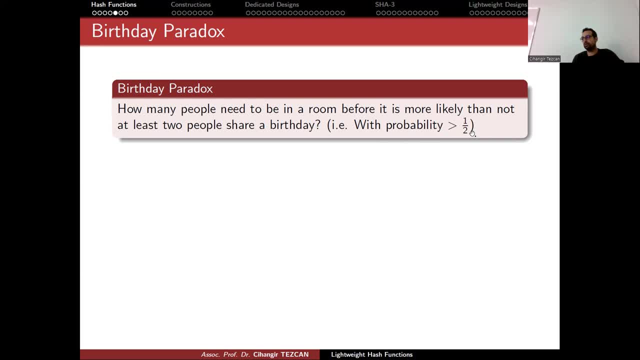 before. it is more likely than not, at least two people share a birthday, right? you know, more than more likely than not, i'm saying with probability, more than one over two. so think about the room. there isn't any people inside. you started to, you know, send people one by one, so after which point on. 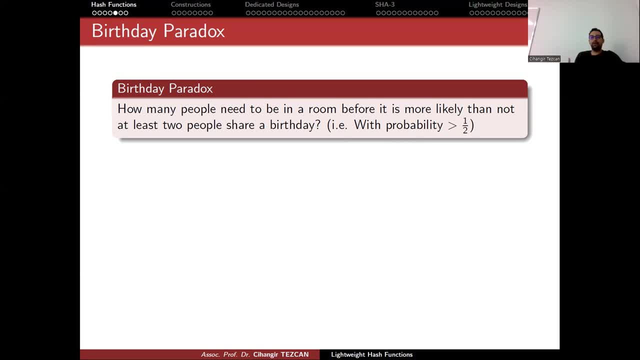 so maybe you know the answer? no, Okay. so people think that you know. since there are 365 days in generally in a year, they think that it should be around 100 or 150 and so on. but I think the answer was 23, okay. 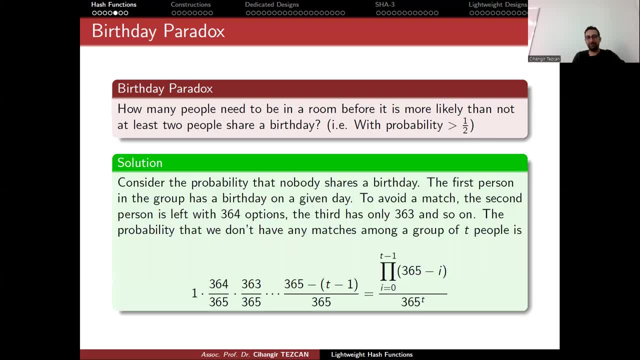 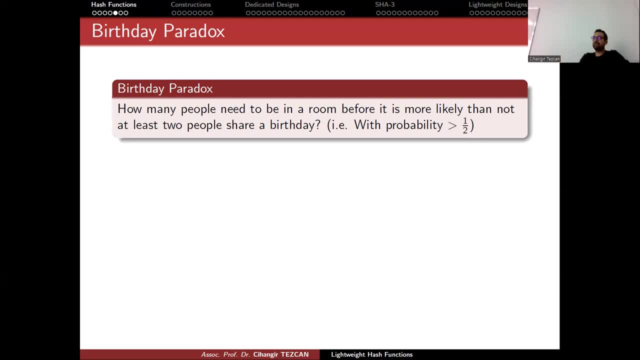 If I'm mistaken, it will be corrected in the slides anyway, but I remember it as 23.. So, since 23 is really a small number compared to the people's expectations, this is why we call it the paradox. Actually, there is no paradox about it. 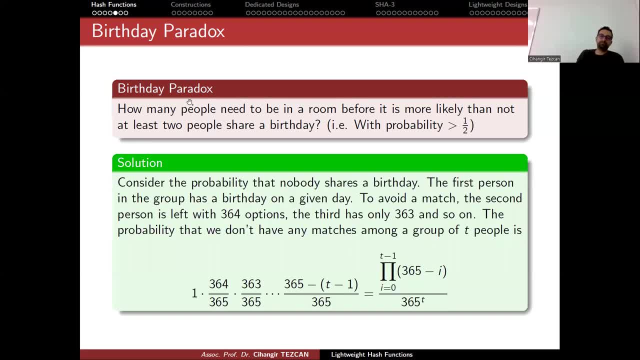 It's just you can calculate it and see it, okay. So how do we calculate it? Consider the probability that nobody shares a birthday, So let's try to calculate this. The first person in the group- this one- has a birthday on any given day, so it is not a problem. 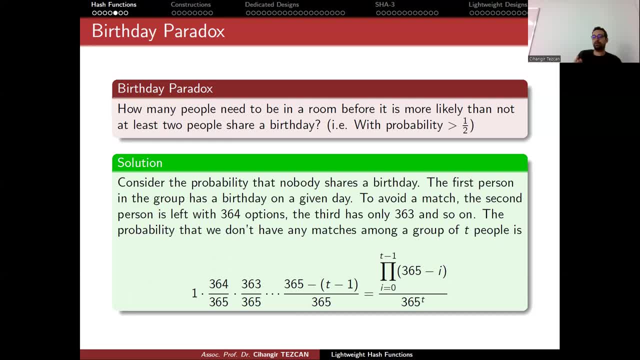 But when I sent the second people, I'm expecting them to not to share a birthday, right? So the probability of this is, you know, there are 364 days left from the whole year, So this is the probability of second person not sharing the birthday with this one. 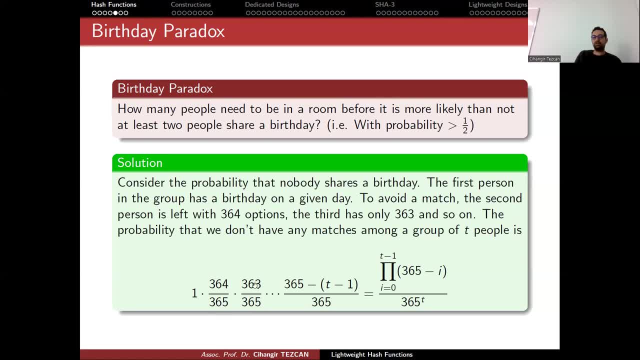 But now you are sending the third person, but this third person should not share the birthday with this one and also this one. So this is something missing. So paradox actually comes from here, because we are limiting your possibilities in a very fast way. So if you keep this, 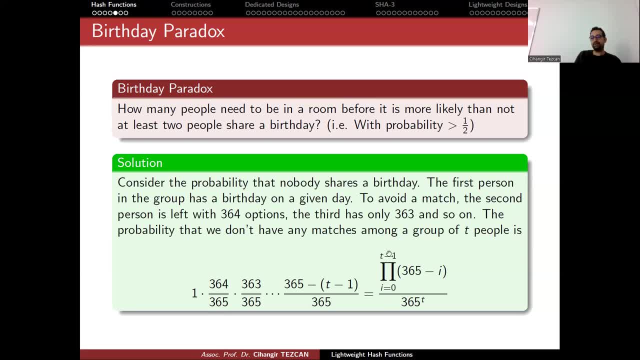 after too many people goes inside the room, this is the you know probability that they are not sharing the birthday. okay, So if this is the property of not sharing it, one minus this number is the probability of them sharing it okay. 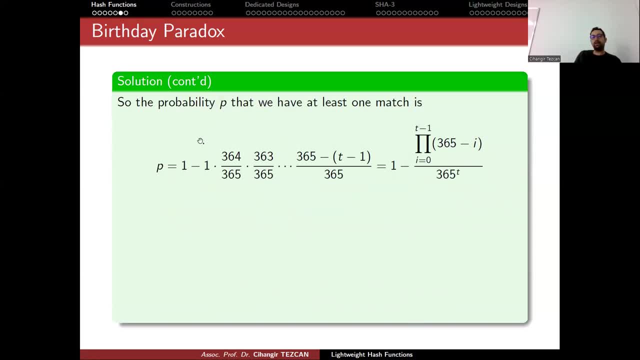 So the probability P that we have at this one match is one minus this, which is one minus this summation and, I'm sorry, the multiplication. Okay, yeah, Calculation shows we have P is larger than to when t is equal to or larger than 23. okay, so, namely, we have probability equals to 0.507. 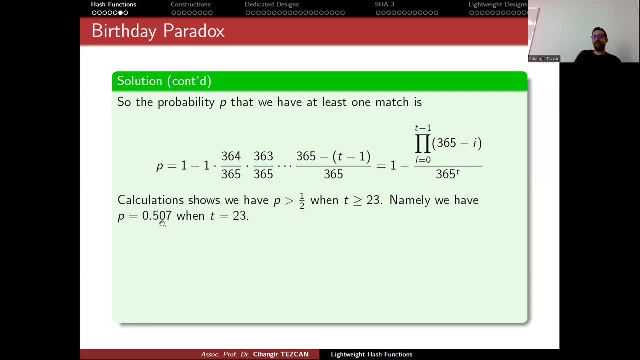 when t equals to 23.. so this is still like the probability of you know, tossing a coin and guessing it. so 23 most probably would not be enough for you. if you're lucky it will be enough. but if you choose, t equals to 30 or something, this probability increases in a really fast way. so if there are 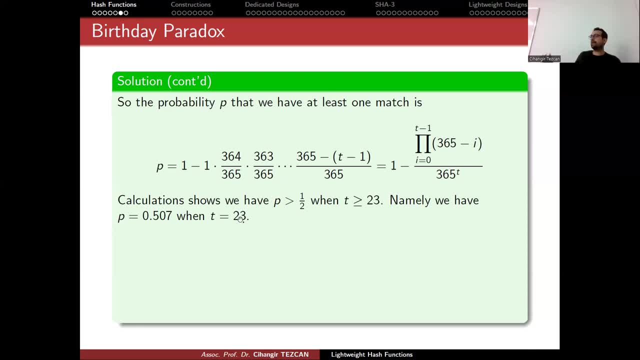 more than 30 people in the room, it is very highly likely that there are more than one people sharing the birthday right? so this is why you know if you are going to try this experiment and you're giving a speech. so currently there isn't 23 people in the room, so i will not try it, but if there are, 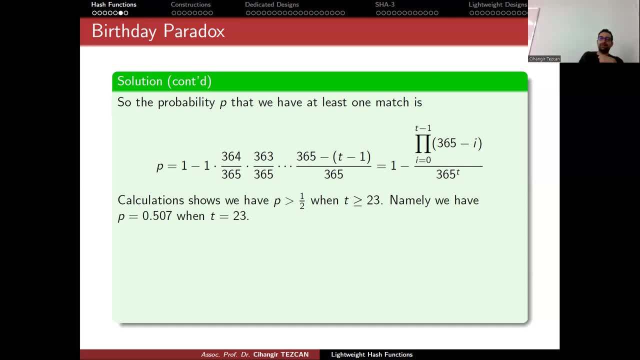 more than 23 people inside the room, you can give it a shot. but if you know already a friend who shared the same birthday with you, and if they're in the room you know always, try this experiment. as a last resort. you can ask their birthday and you know. 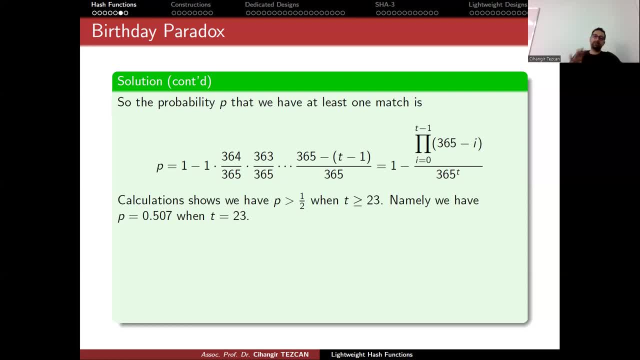 this because this is what i did in the previous years, because the head of department of cryptography shared the same birthday with me, so i asked him in the last, as the last result- and you know, always find the second person okay. so why this is important, or why this is related to the 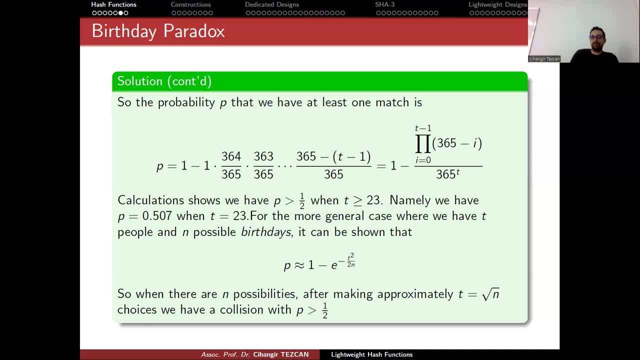 you know, finding a collision. for the more general case where we have t people and impossible birthdays, it can be shown that probability is approximately equivalent to y minus e, to the power minus t squared divided by 2m. okay, of course this is an approximation. so when there are n possibilities, after making 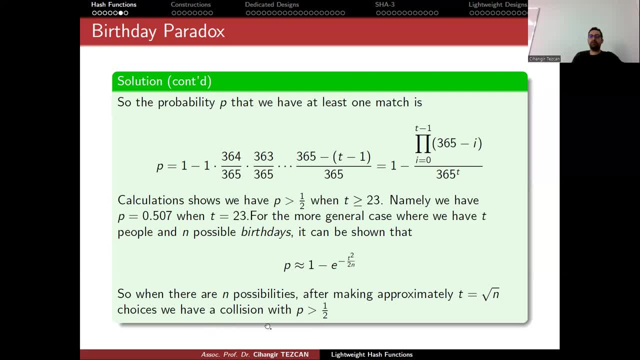 approximately t equals the square root of n choices, we have a collision with probability one over two. this is why, in our case, uh, by m possibilities, in our hash function, we have two to the m possibilities. once you take the square root of it it becomes, you know, two to the n over 2.. of course i'm saying 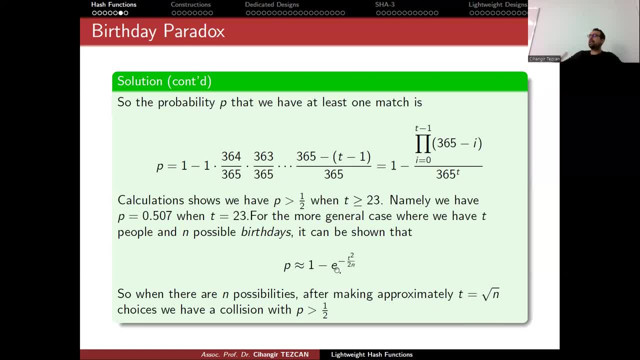 approximately, because this approximation works when n is really large. so if you- because if you focus on our example, we have 365 days- if you take the square root of it, it wouldn't give you 23 because there is actually multiplication with the constant here. but I removed that constant and said approximately instead. for huge numbers, that constant is not that. 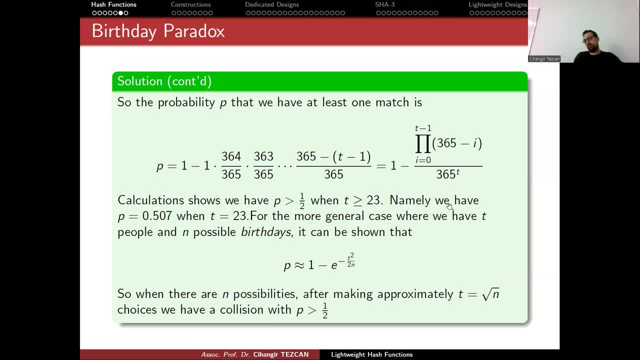 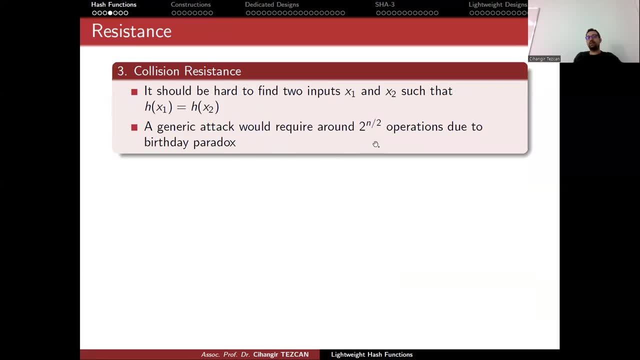 important, but for small numbers, of course, it would be important, but anyway, this is why, if you go back to the collision resistance, this is why a generic attack would require this manipulation. so this is important because this actually gives you a security upper bound. so, if you choose any, 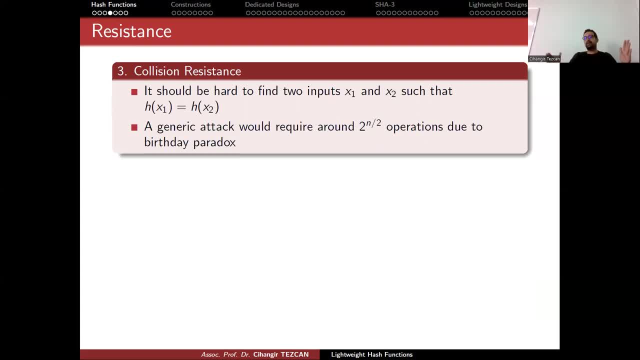 cost of 128, like MD5, then this means that a generic attack will require 2 to the 64- hash function operations, trials, and 2 to the 64 was a huge number 10 years ago, but it is not that huge today because we have a lot faster CPUs, GPUs or ASICs, okay, so this is why we increased this n. 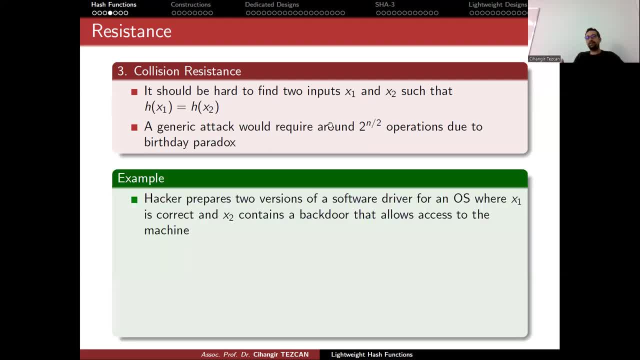 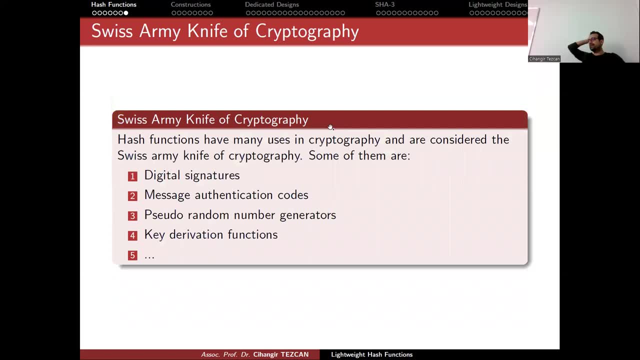 to 256 years ago. okay, so this is why you should should use something shorter, and I will actually mention all of them when we talk about dedicated designs. okay, Like MD4 or MD5.. Okay so, let's finish this with the last slide. I said that